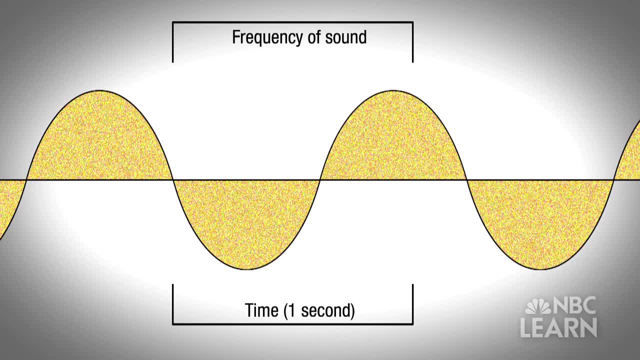 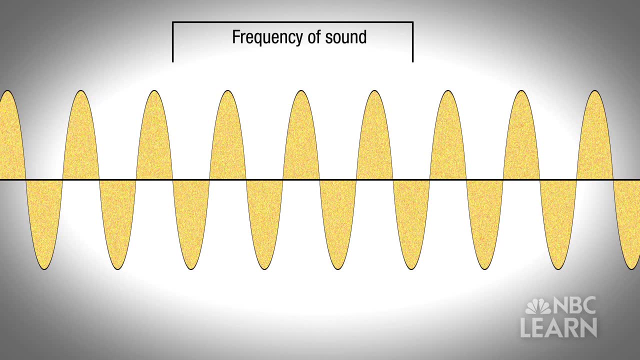 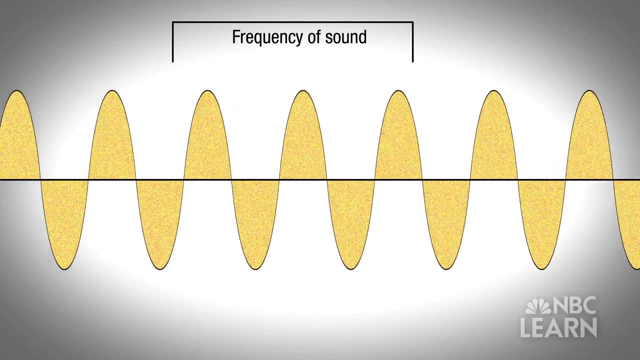 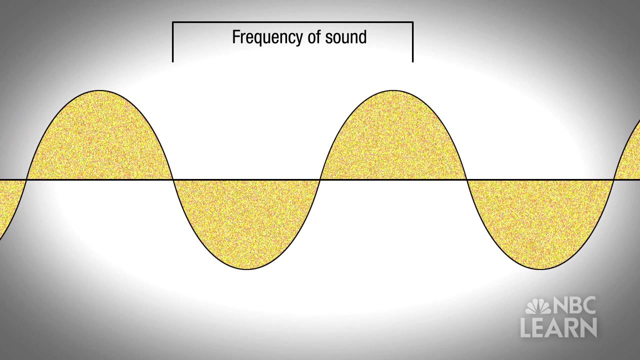 The frequency of a sound wave determines its pitch, or how high or low the sound is. Sound waves caused by faster vibrations have higher frequencies and make higher-pitched sounds like birds chirping. Sound waves caused by slower vibrations have lower frequencies and make lower-pitched sounds like a foghorn. 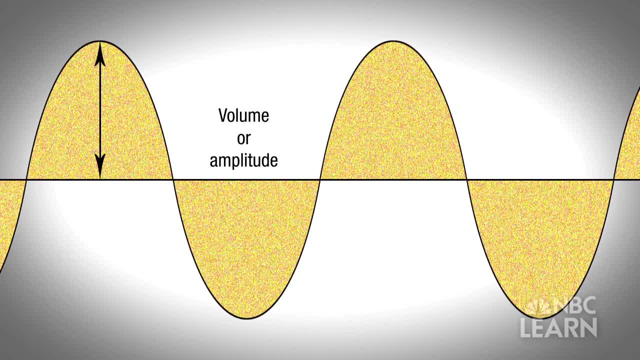 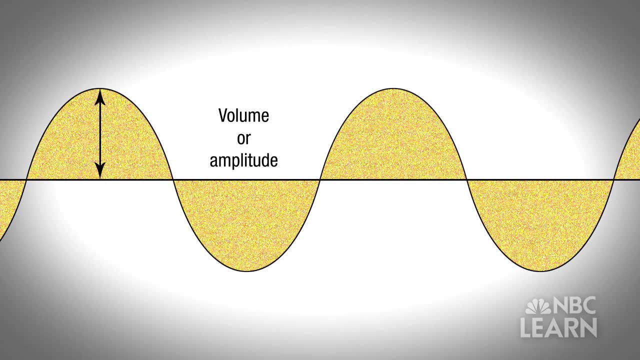 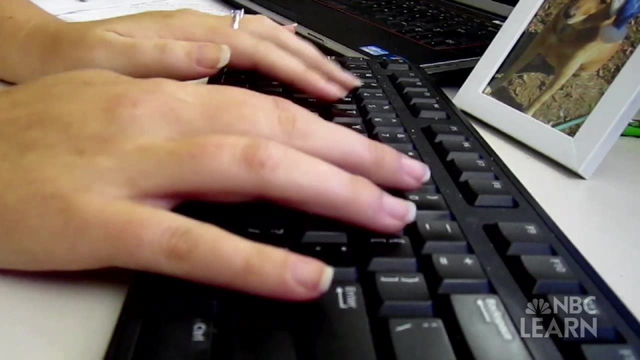 Volume is how loud or soft a sound seems to your ears. Volume is determined by the amount of energy a sound has. For example, a sound like thunder has more energy and sounds louder to your ears. The sound of typing has less energy and sounds softer. 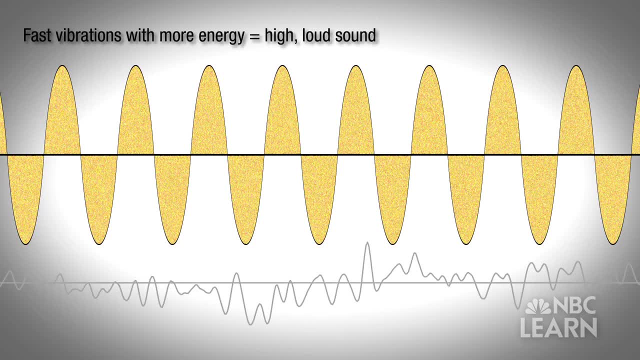 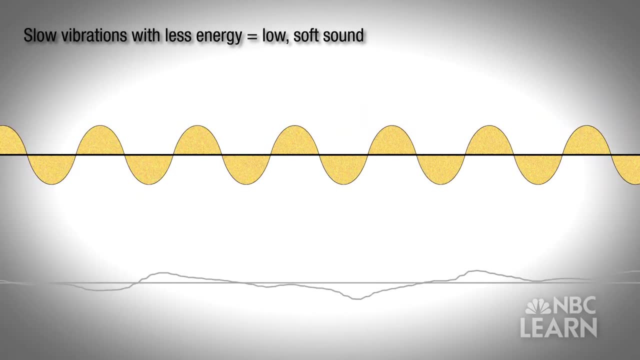 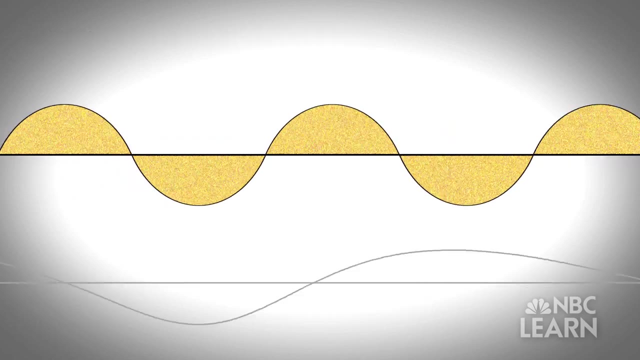 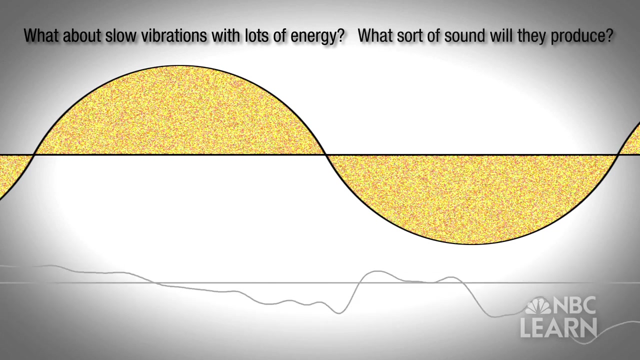 Fast vibrations with more energy will produce a high, loud sound, And slow vibrations with less energy will produce a low, soft sound. What about slow vibrations with lots of energy? What sort of sound do you think they will produce? That's right, They will produce a low, loud sound. 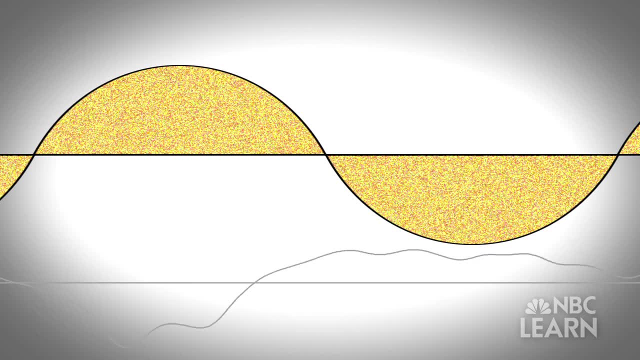 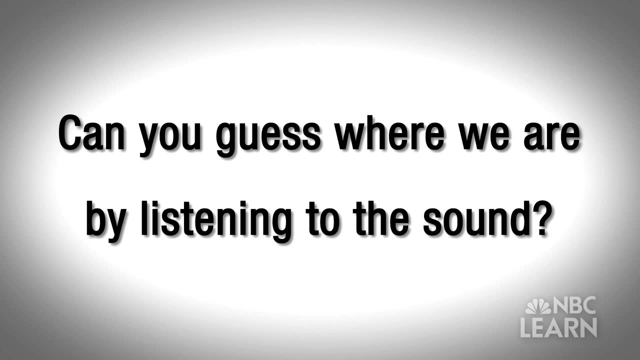 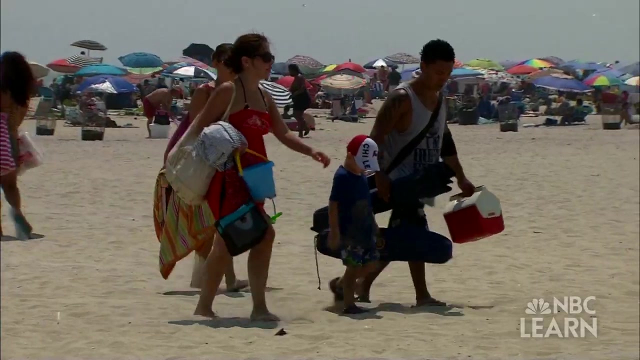 To demonstrate just how important sound can be to our lives. let's play a game. Can you guess where we are by listening to the sound? Did you guess it? We're at the beach. Sound can give you hints about what's happening around you, even if you can't see. 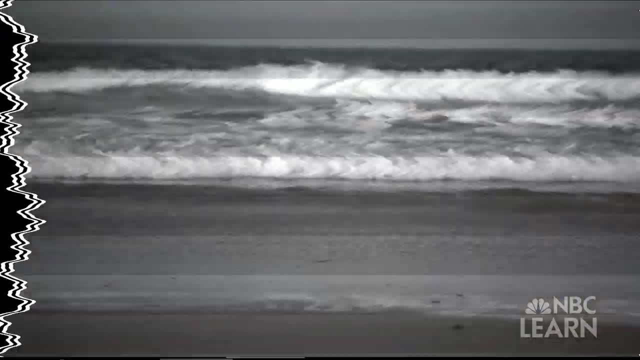 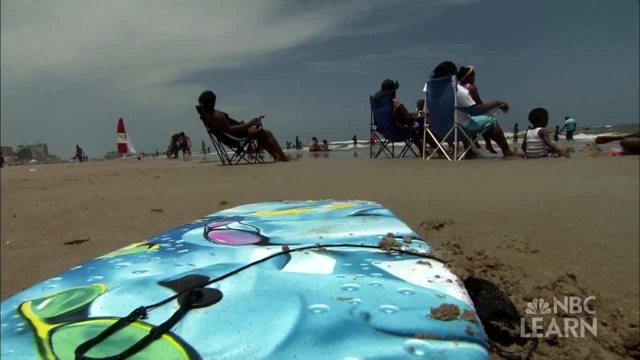 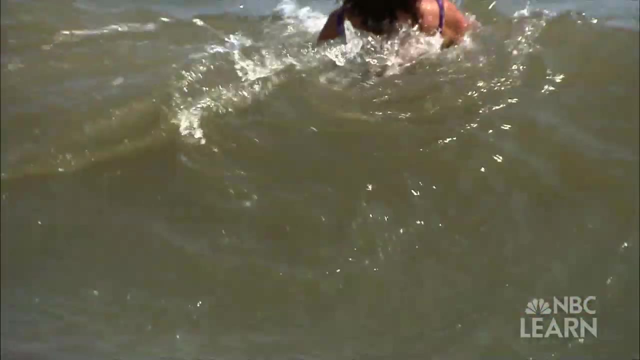 Let's look at the same example in a different way. Here's a video of the beach without sound. Now let's have our video editor, Brian, add in the sound of the waves crashing, then the seagulls, then the children playing in the sand, and it all comes together. 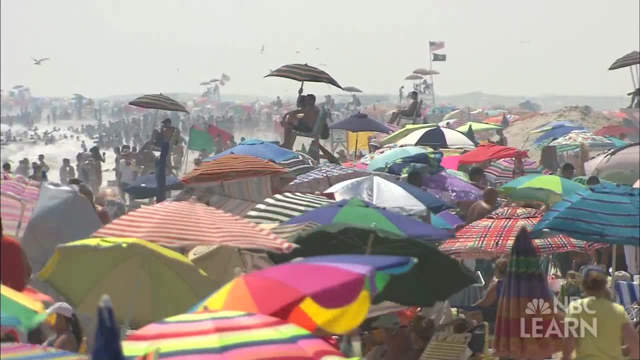 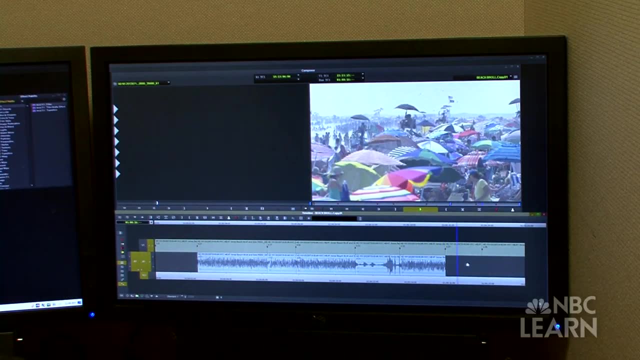 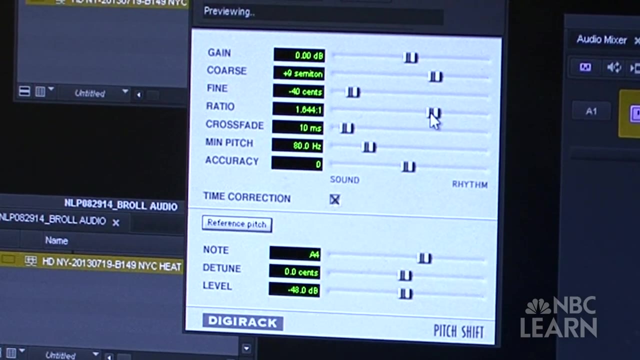 To make this happen on video, Brian carefully added the sound into the video at the right volume. Video and film editors like Brian can also change the way things sound. They can take the pitch of my voice and make it sound very high and silly or very low and spooky.